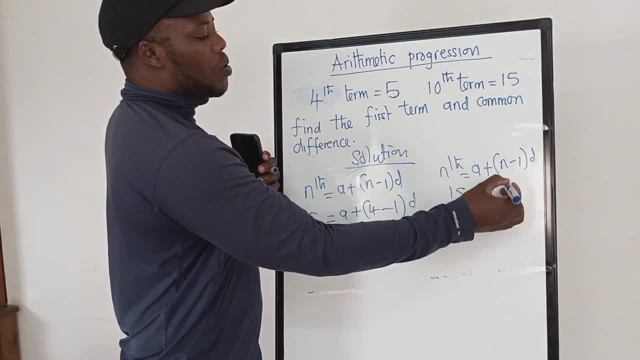 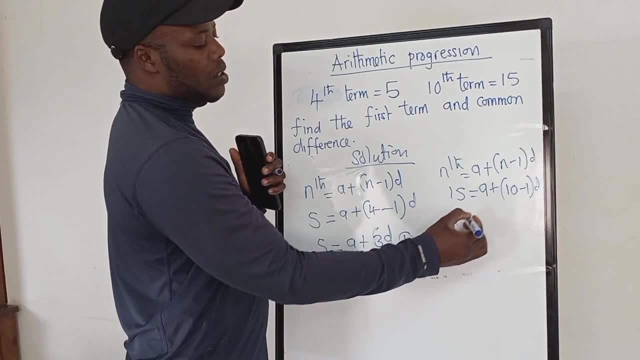 Put 15 here. a is what we're looking for. On n, put a 10 minus a 1 and a d there. Okay, so you simplify, You remain with 15.. It's equals to a plus nine d. This is nine d, Okay. 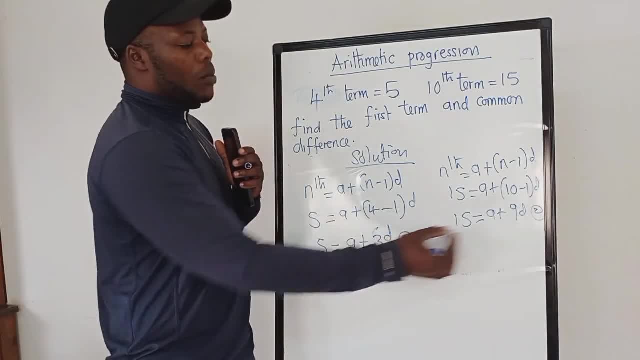 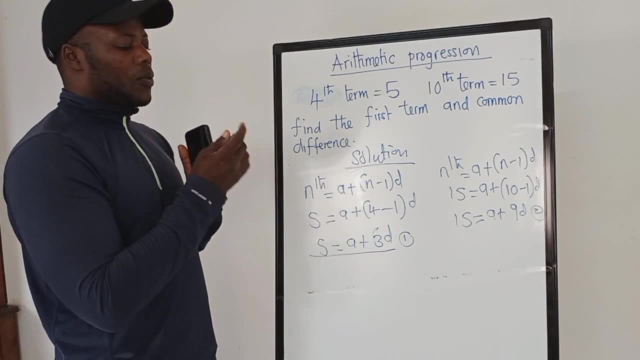 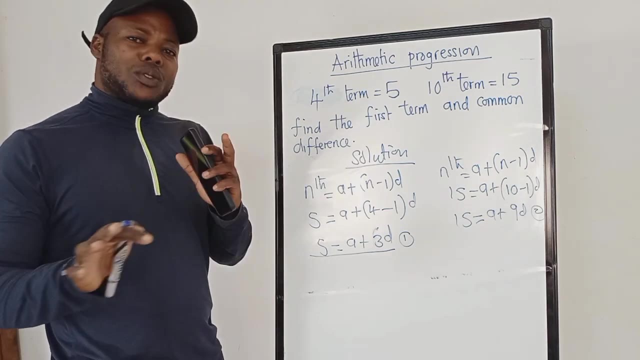 so we'll call this equation number two. This is equation number one, number two. So once we reach this point, we can solve these two equations simultaneously. Okay, so if you don't know how to solve the simultaneous equation, you just have to know how to solve the simultaneous equation. 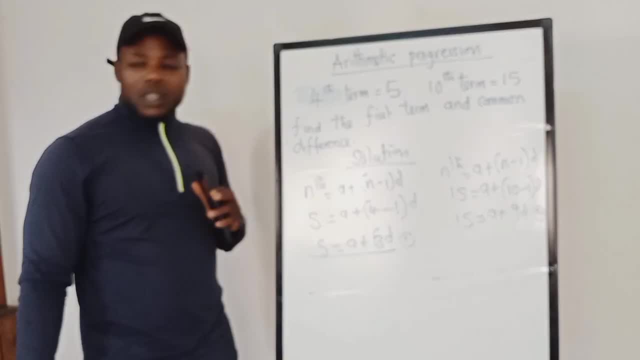 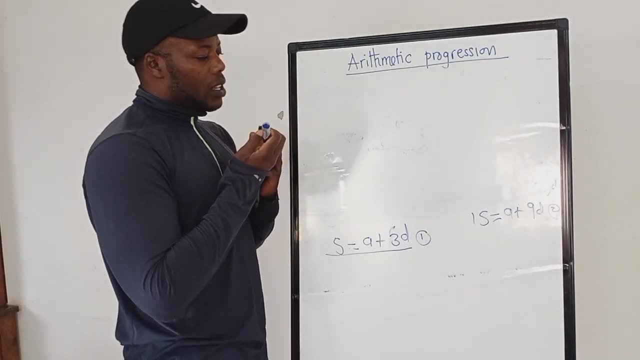 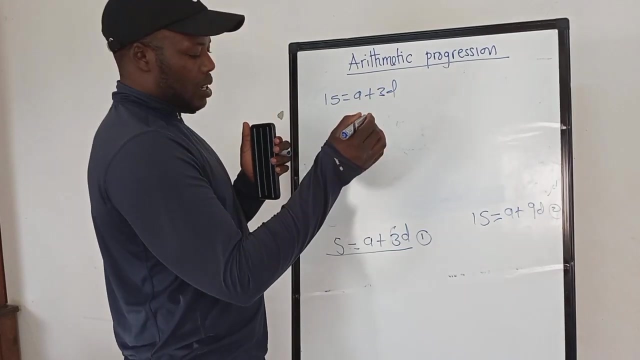 So check on my videos. I think I did a video on simultaneous equations, on how to solve simultaneous equations, So we've got these two equations that we are solving simultaneously. So we have 15 is equals to a plus three d. Sorry, this is five, Not 15,. 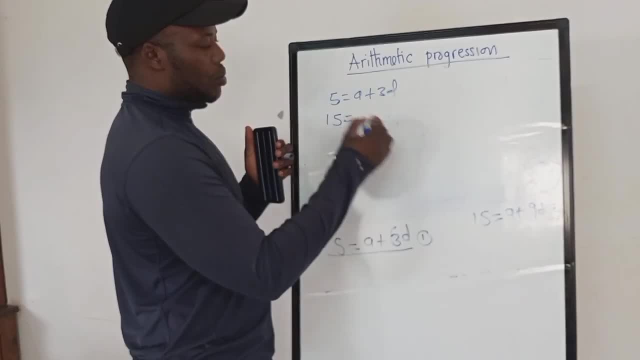 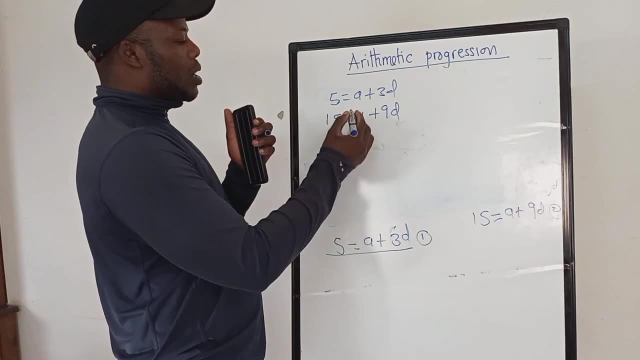 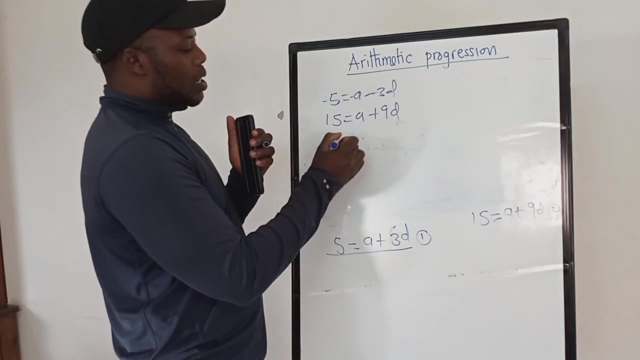 five, Here it's 15.. It's equals to a plus nine d, And we need to solve these two equations simultaneously. So what we can do here? we can just put a negative here, negative here, and also change this to a negative. So here we have a: 10 is equal to here. 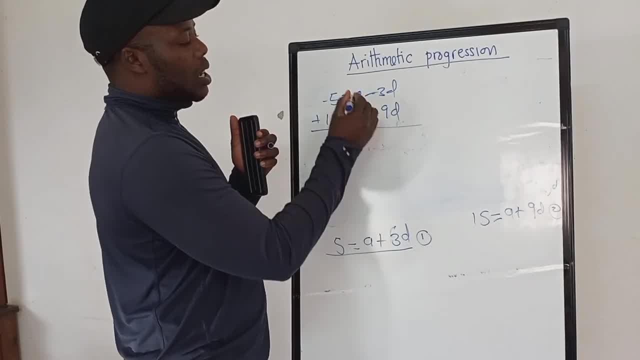 We have a 0, because 1. We're adding them actually A negative a plus a is just a zero. Here. with a 10 can we can solve them again with a maxim. So here we have a 10. It's equals to 1,. we have a 0 because 1. We're adding them actually A. negative a plus a, it's just a 0.. Here we're adding them. actually A negative a plus a, it's just a zero, Because one we have ten. This is we have a value of t plus zero. So here, if we solve theный, we can solve the them. Now we have. 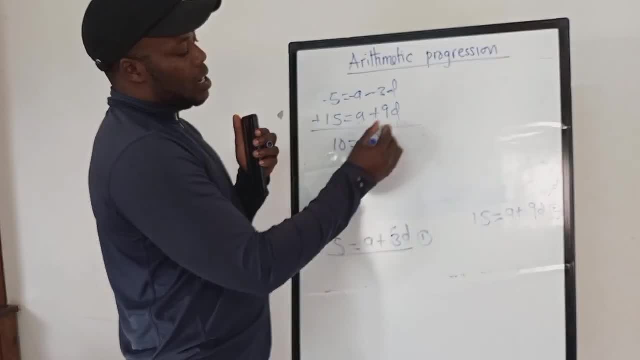 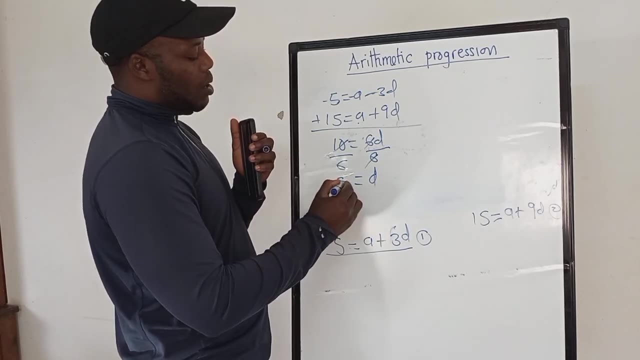 So here we have a 60D, And when we solve- we work out solving for D- our D will be equal to 5 over 3.. This is our D: 5 over 3.. So we have found a common difference. 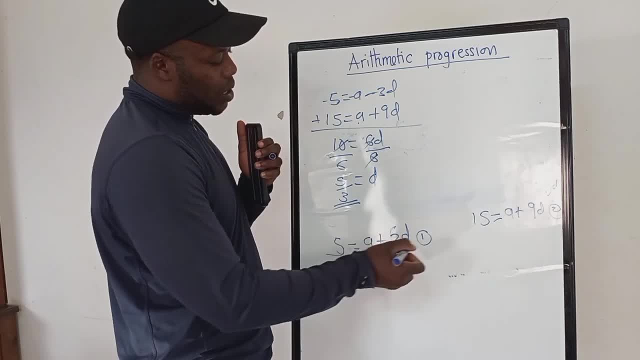 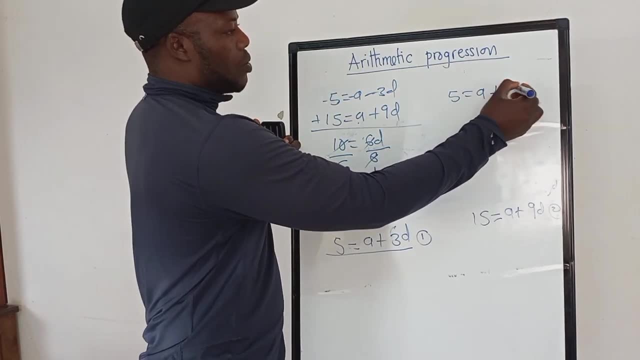 Now to find the A. we can get any of the equations, either this one or this one, So I'll go with this one. I'll say 5 is equal to A plus 3D. 5 is equal to A plus 3 on D. 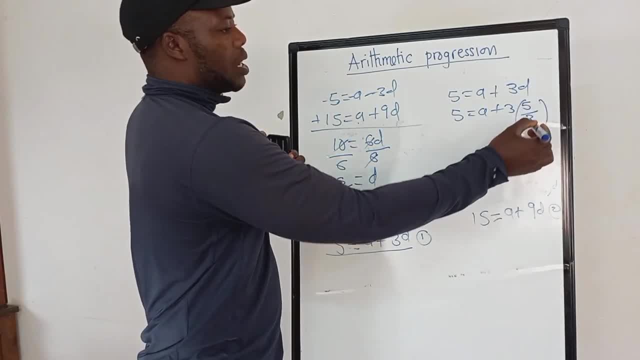 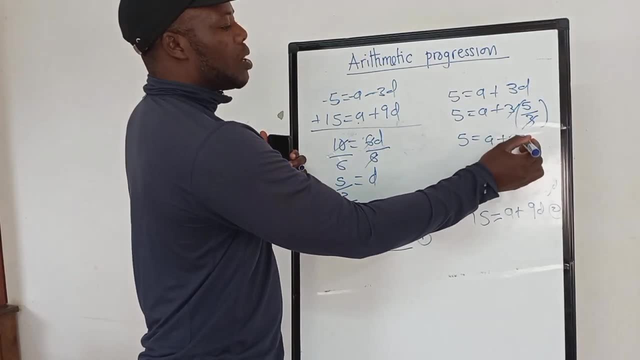 I'm putting a 3,, I mean a 5 over 3 here. So this and this will cancel or remain with 5A plus 1, actually 5, because this 3 and 3 have canceled And when you group the like terms it will be like this: